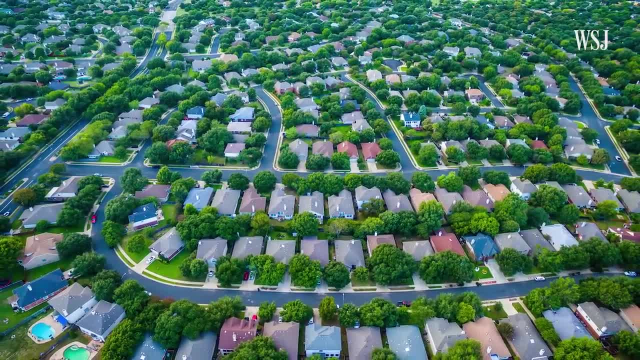 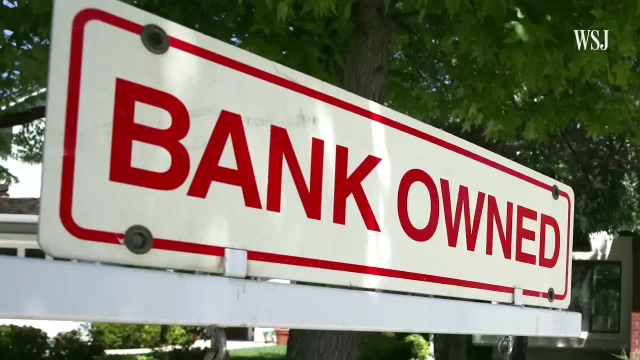 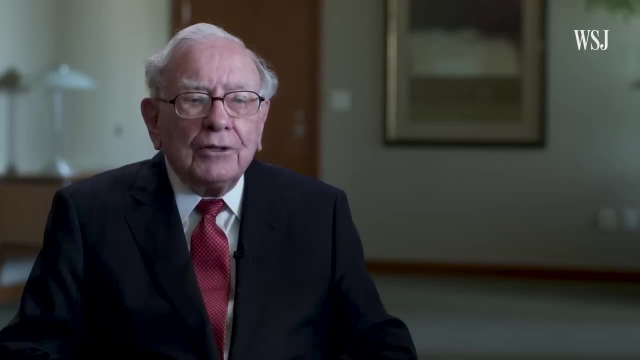 50 million people had mortgages roughly at that time out of 75 million homeowners. When that bubble burst, it hit home to probably 40% of the households in the country. These people would have mortgages on their houses And fear spread in the month of September 2008 at a rate that was like a tsunami. 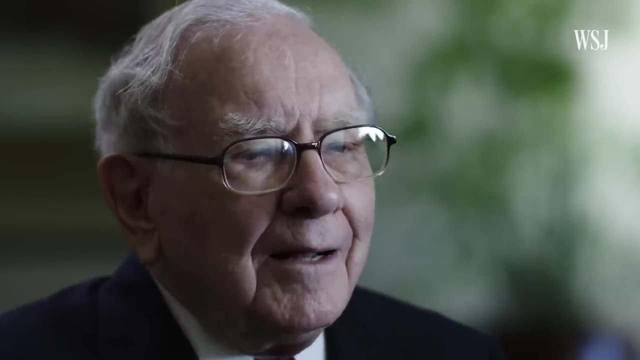 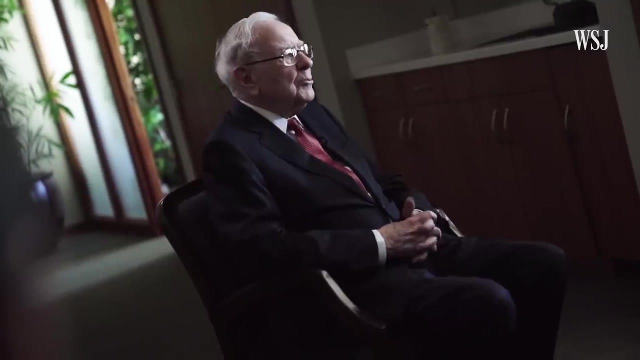 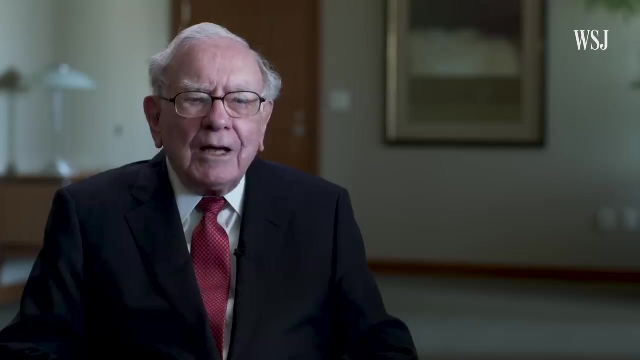 Who do you hold responsible for that? Bubbles are always hard to ascertain the originators of. There really aren't any originators. Everybody got caught in, Some were foolish, Some were crooked, Some were both, But you had a. 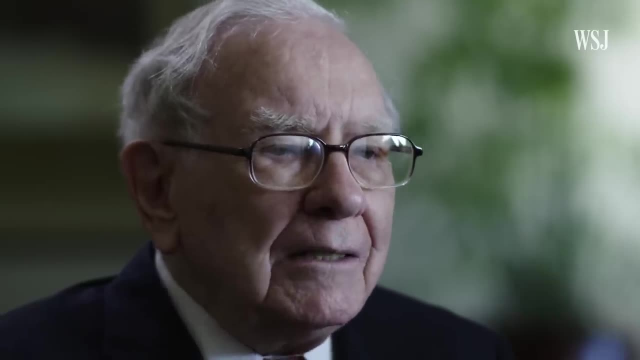 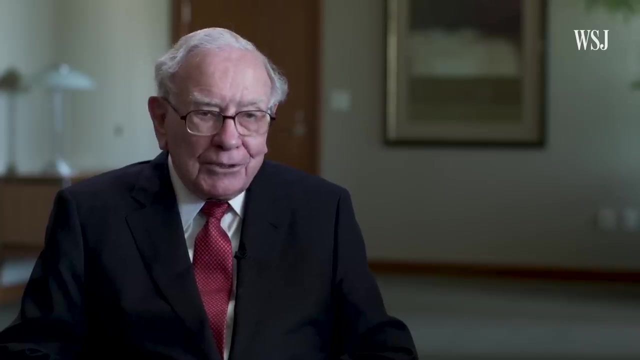 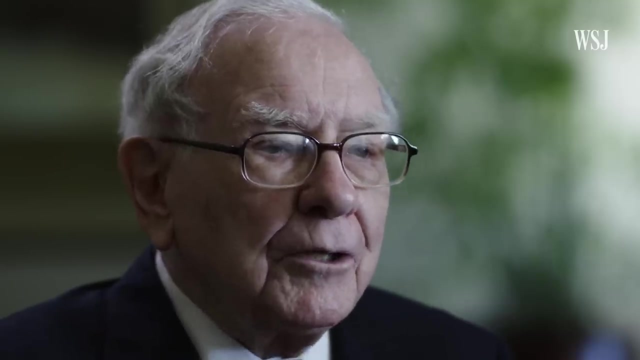 Mass illusion that it could go on forever. You had Wall Street firms participating, You had mortgage originators participating, But you had the public participating And it was. you know, it was a lot of fun. I mean, it was like going to Cinderella, going to the party. 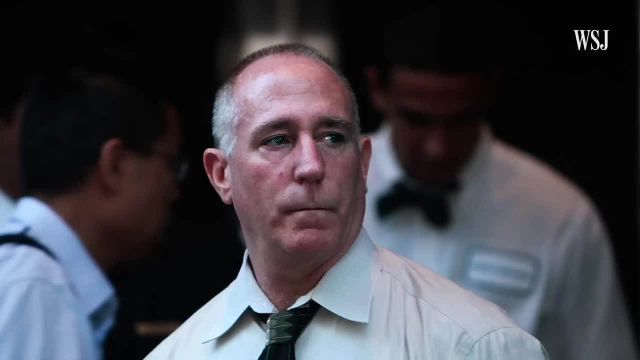 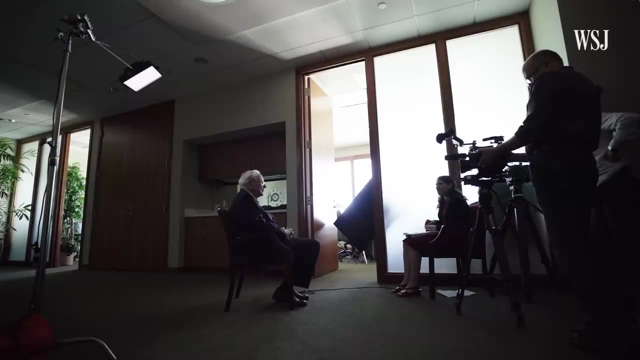 I mean, it was all going to turn to mice and pumpkins at midnight, But nobody wanted to leave until one minute to midnight And the rush for the door couldn't be handled. What, for you, were the? The lessons you learned from 2008?? 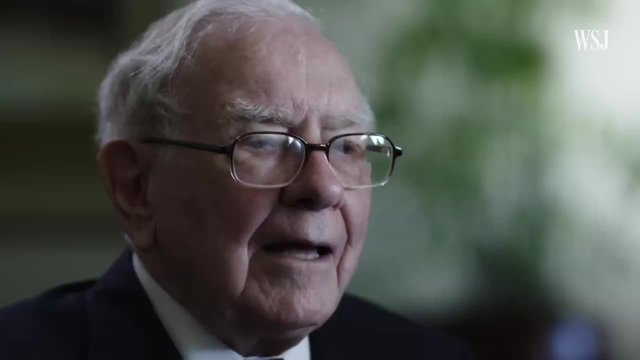 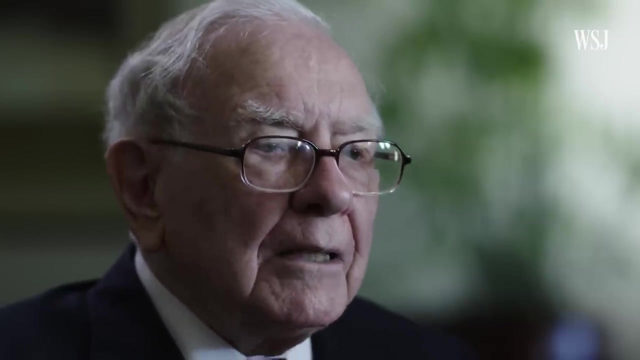 I didn't really learn any new lessons in 2008 or 9.. And I had emphasized to me some of the things that I'd always believed That you do need somebody who can say: well, do whatever it takes. The US government had to do the right things. 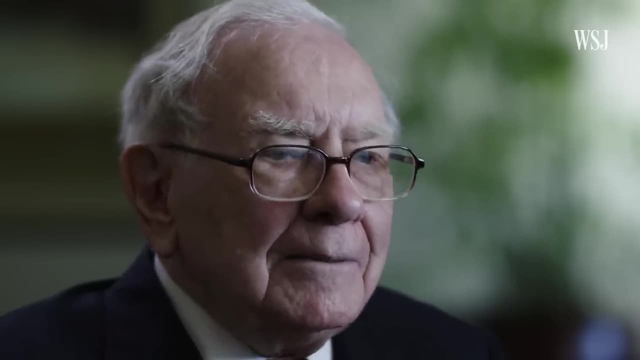 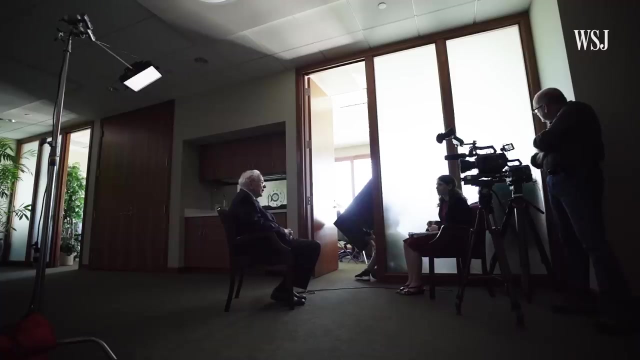 Not perfect things, but generally the right things, starting in September, And they did a fantastic job actually of getting the train And getting back on the tracks. There was still damage for a long period thereafter, But it was really important to have fast action at that time. 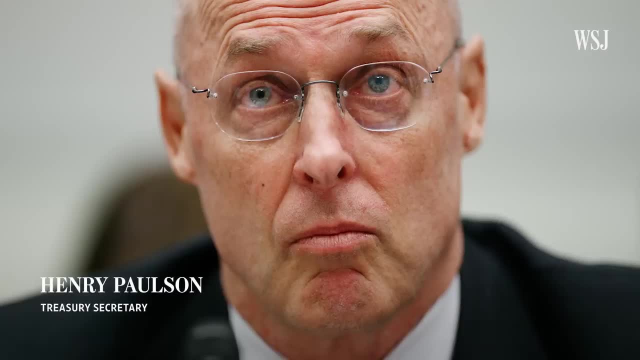 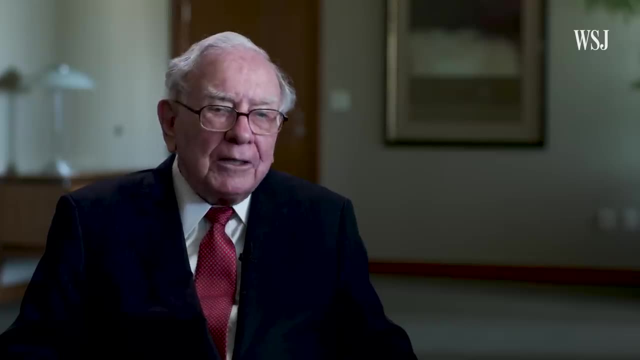 And we were very fortunate we had the leaders we did. If we'd had people who waited for all the information to be right or for committees to work or you know that sort of thing, it would have been far, far worse.